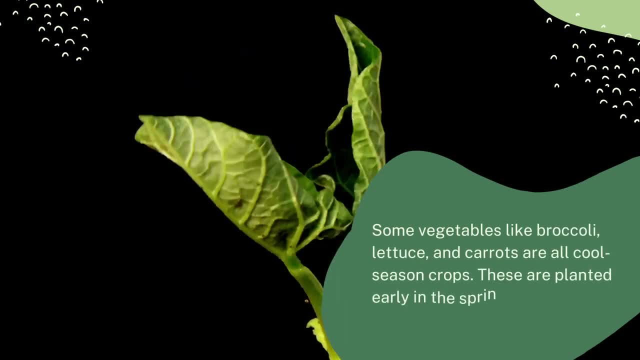 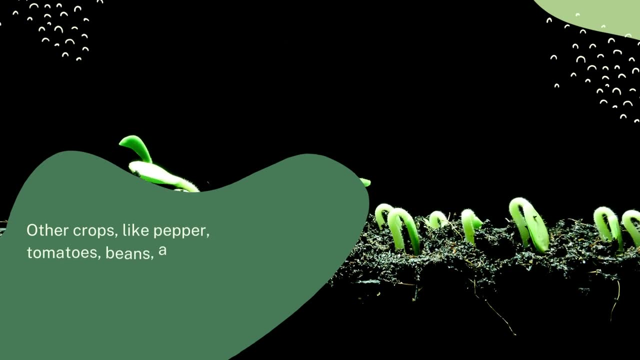 and carrots are all cool season crops. These are planted early in the spring and can't tolerate heat. Other crops like pepper, tomatoes, beans and corn are warm season crops. They grow in the heat of summer until the fall frost kills them. 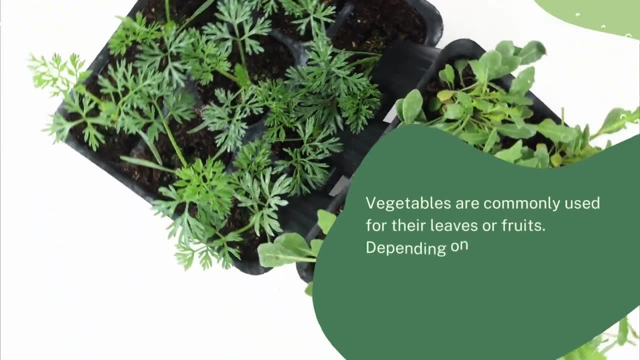 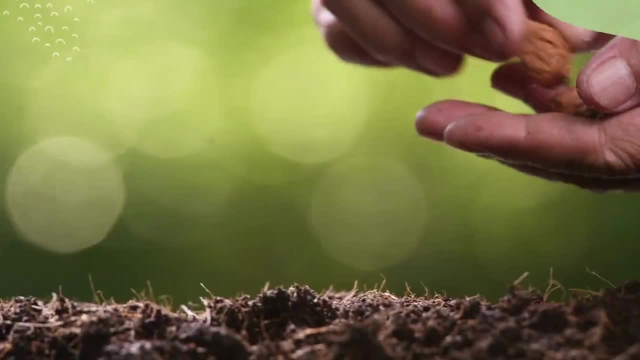 Vegetables are commonly used for their leaves or fruits. Depending on the vegetable type, you can tell what plant it is by looking at its leaf and knowing its variety, The time of the year the vegetable is growing. In temperate zones, early crops are planted in. 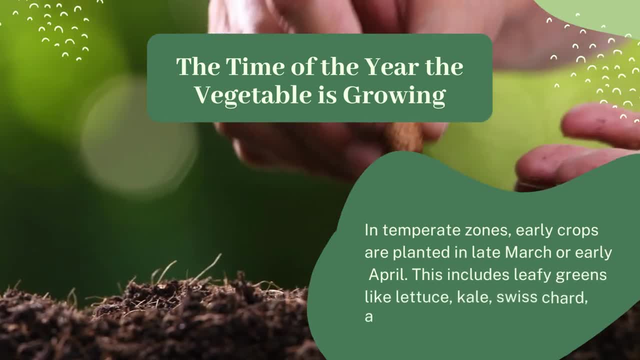 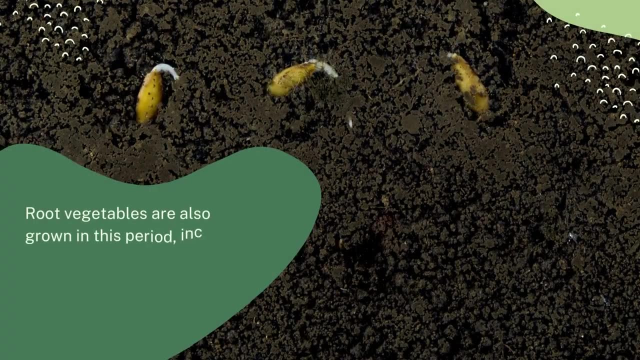 late March or early May. The time of the year the vegetable is growing is the time of the year, the early April. This includes leafy greens like lettuce, kale, Swiss chard and spinach. Root vegetables are also grown in this period, including onions, beets, carrots and radishes. 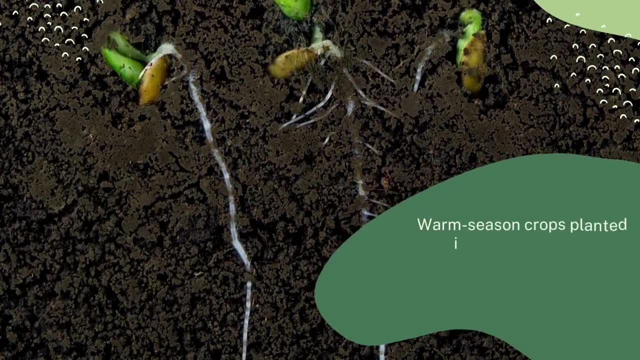 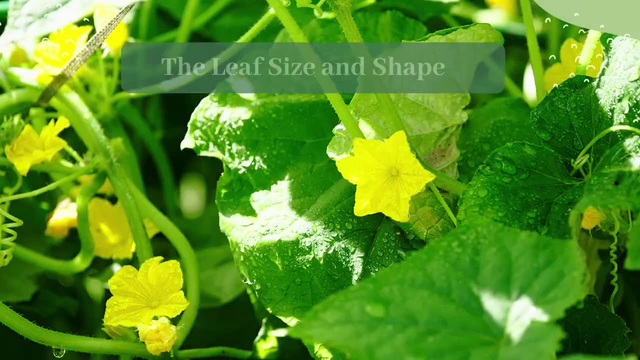 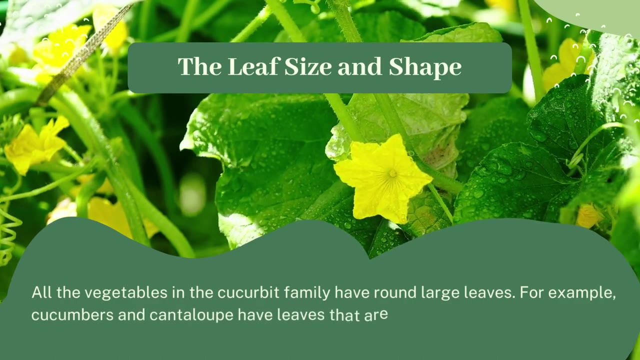 Peas are also planted at this time. Warm season crops planted in June and July include melons, peppers, tomatoes and eggplant. The leaf size and shape: All the vegetables in the cucurbit family have round large leaves. for example, cucumbers and cantaloupe have leaves that are 3 to 4 inches across. 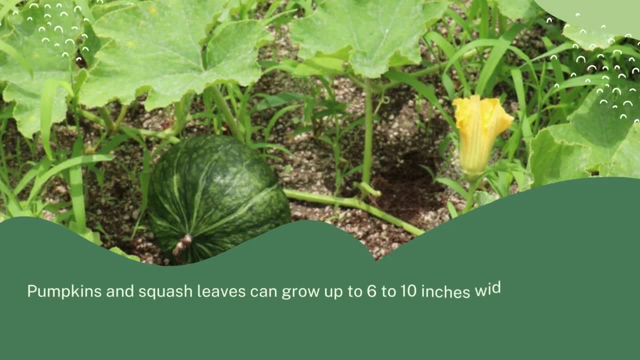 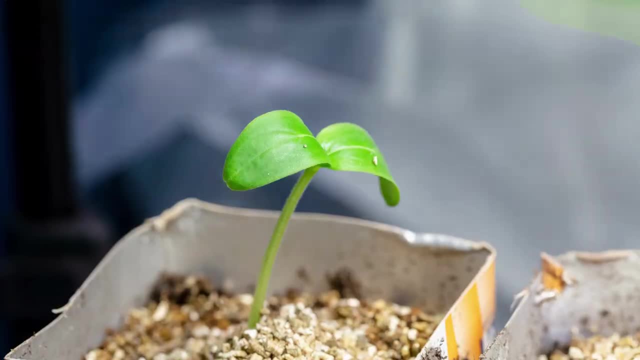 Pumpkins and squash leaves can grow up to 6 to 10 inches wide. Beans, tomatoes, eggplant and peppers have leaves that are 2 to 3 inches wide. The leaf formation Fruit-forming vegetables like peppers, tomatoes, eggplant and beans. 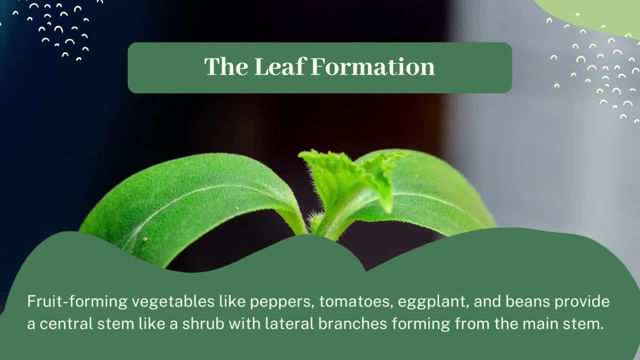 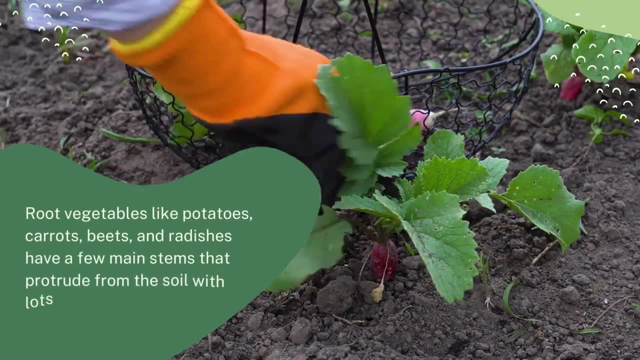 provide a central stem, like a shrub, with lateral branches forming from the main stem. Root vegetables are also grown in this period, including onions, carrots and spinach. Vegetables like potatoes, carrots, beets and radishes have a few main stems that protrude. 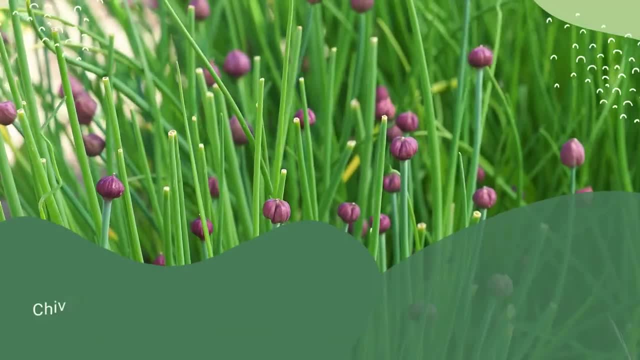 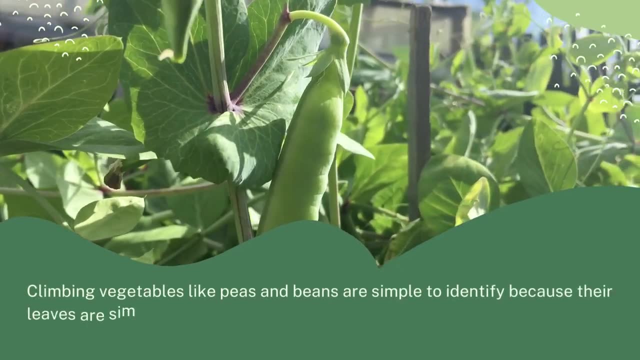 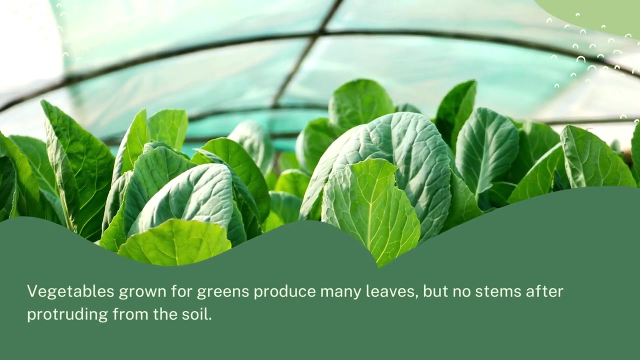 from the soil with lots of leaves. Chives and onions have tall, spear-like leaves that are distinct in shape. Climbing vegetables like peas and beans are simple to identify because their leaves are simple. Vegetables grown for greens produce many leaves but no stems after protruding. 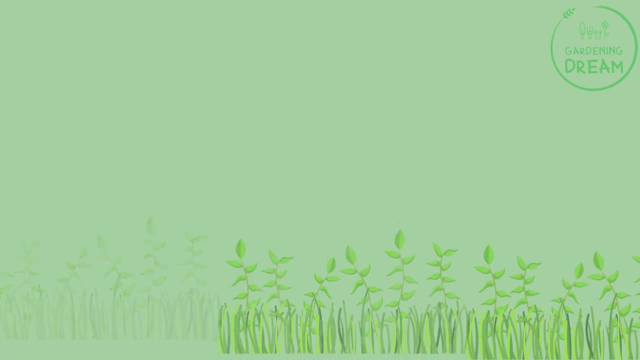 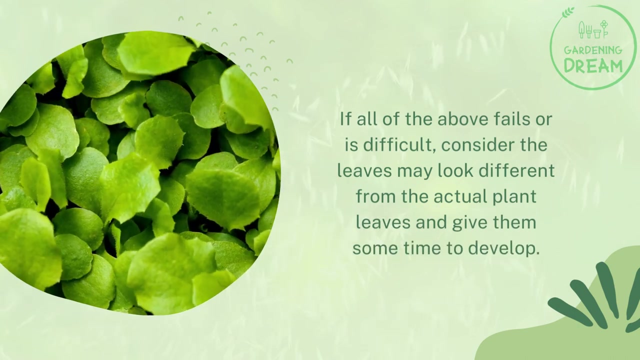 from the soil Use considerations. If all of the above fails or is difficult, consider the following. If all of the above fails or is difficult, consider the following: Consider the leaves may look different from the actual plant leaves and give them some time to.